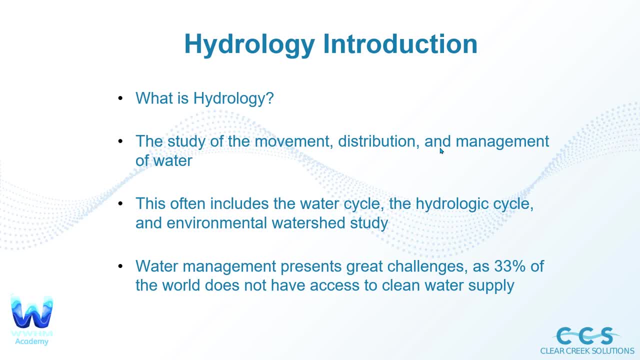 great challenges, as 33% of the world does not have access to a clean water supply. especially as the population of the world continues to increase, access to that clean water supply is going to be very crucial. It's going to be very critical. We want to make sure we can get clean. 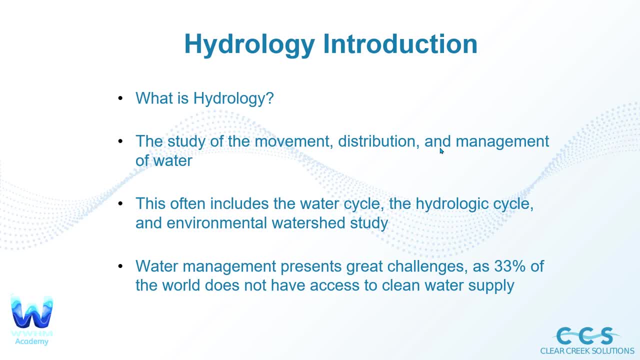 water to everyone, have stormwater mitigation methods. that keeps everyone safe, keeps economic damage from occurring and, just overall, makes the world a better place. That's kind of the idea of water resources engineering. But clean water supply and environmental engineering, ensuring that that water is filtered correctly and safe for the general population- is a big deal with 33%. 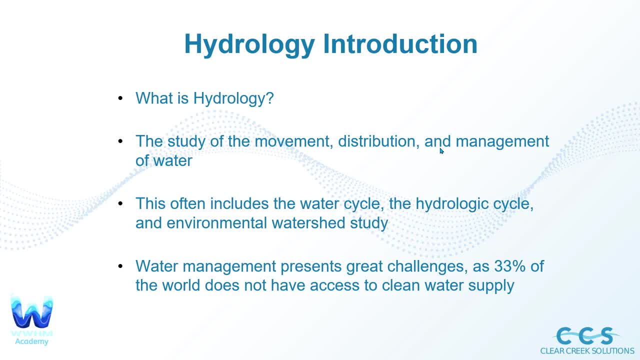 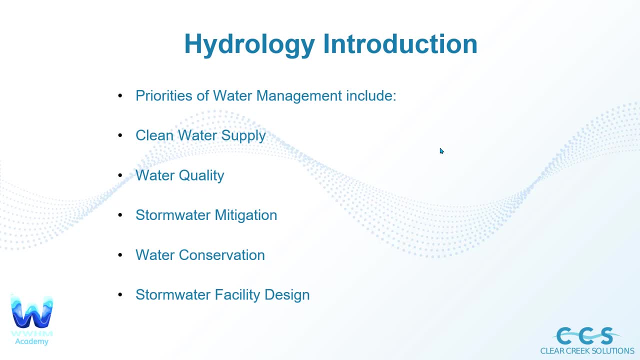 lacking that access. This field is only growing and getting more important, So some of the priorities of water management include making sure everyone has access to that clean water supply- overall water quality. also making sure that there's not too many erosion in our streams. So if we have too much runoff from a site, there's too much erosion because erosion 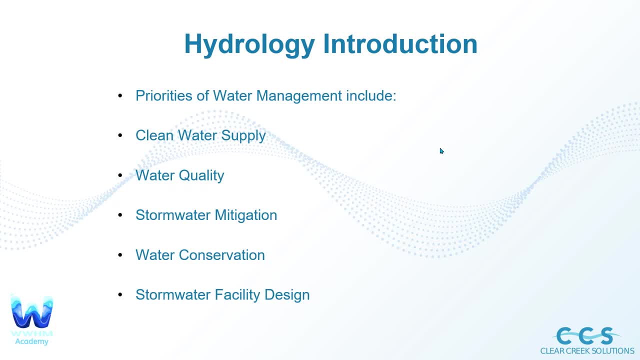 does occur in natural streams. If there's too much, then it's going to start to erode, get in our streams and reduce the water quality of our streams, And we don't want that to happen. Stormwater mitigation, making sure when it does rain, when it does run off, from these various 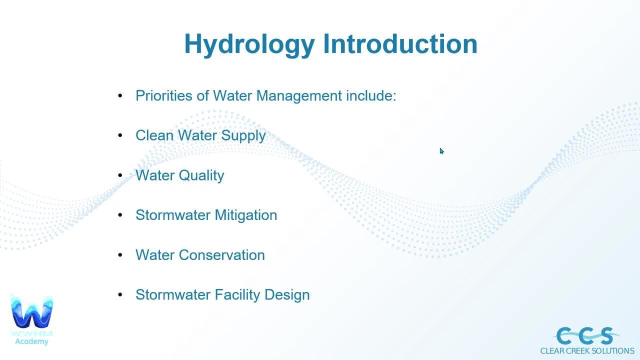 sites, that it goes to the right places, that it's treated, it goes to detention facilities and it's stored correctly and managed correctly. Water conservation in some areas, especially that do not get lots of rainfall, making sure they have access and they conserve that clean water. 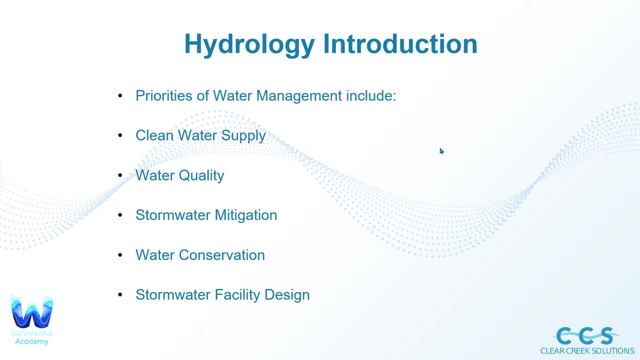 So when they get the rain, maybe during the winter months, they're able to conserve that water and then use it all through the summer. So that's gonna be really important. And then, of course, stormwater facilities design, such as retention ponds, bioretention and various facilities like. 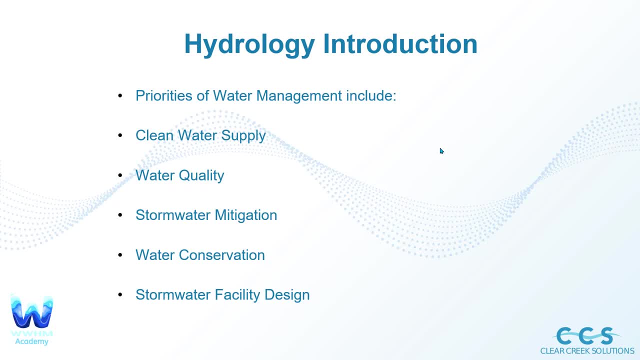 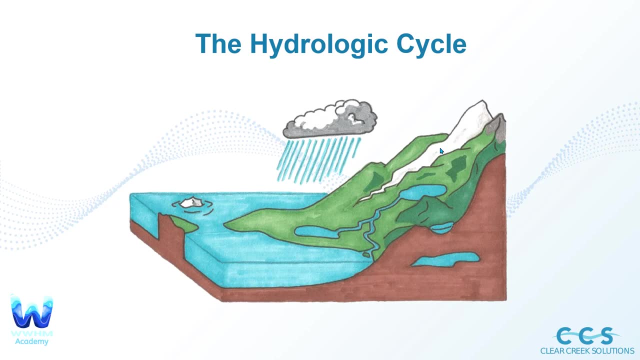 this: they design those facilities for the future, for stormwater mitigation. So let's talk about the hydrologic cycle. You're probably very, very familiar with the water cycle, but the hydrologic cycle is a little more nuanced, but very similar We're. 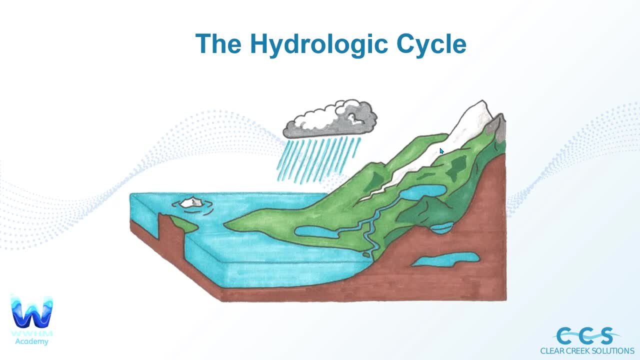 going to get into it, but basically rain is going to fall on a site or on an area. What happens to that water? Well, it's going to infiltrate, It's going to run off the surface, It's going to evaporate into the atmosphere, right? So this is going to give us a good idea of the 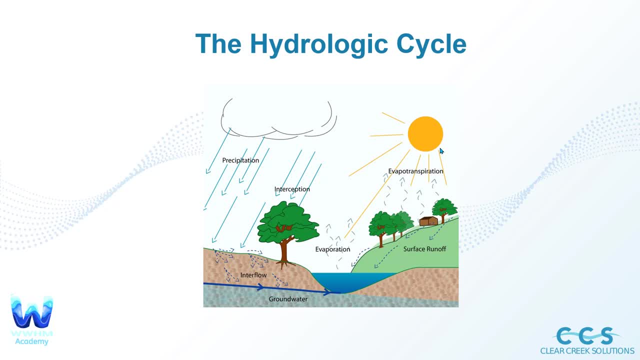 water cycle. So we have precipitation. Some of that is going to intercept into the tree leaves and the actual natural occurring plants in the area. Some of it's going to run off. Some of it's going to become interflow. Interflow is shallow below ground runoff or water, And then some of 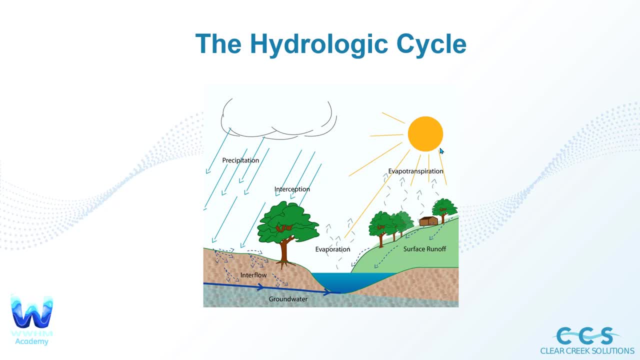 that's going to become groundwater, real deep groundwater in the surface. Some of that water will eventually evaporate back into the atmosphere And then, when it evaporates off these plants where this water was intercepted, that's called evapotranspiration, And if you look on the far right here, that's what's called surface runoff. The water will just 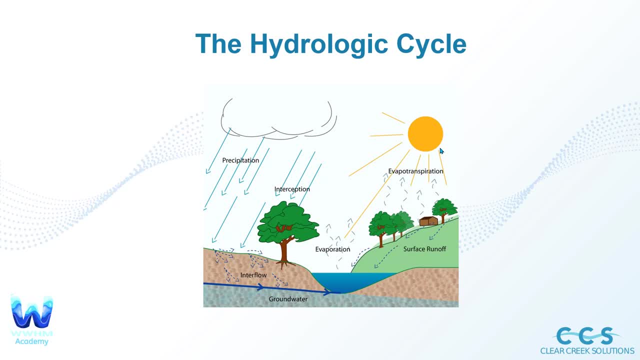 run off straight from the surface. If the soil is impervious, it's too saturated, it'll run off right into the lake here and then basically evaporate, And that is the hydrologic cycle. Our key as hydrologists, water resources engineers, is to track all that water through the hydrologic cycle and 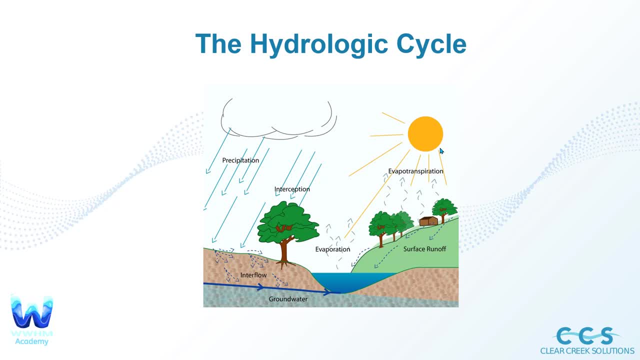 make the best use of it. Make sure the amount that needs to be returned to nature is returned to nature to continue the cycle, The amount that we need to use for other methods, such as drinking, and the amount that needs to get treated for certain natural environments. So that is the 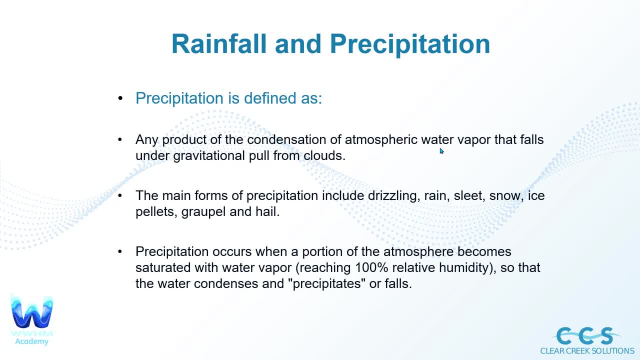 hydrologic cycle. So let's talk about rainfall and precipitation. Precipitation is defined as any product of the condensation of atmospheric water vapor that falls under gravitational pull from clouds right So rain, or I'll go over all the different types of precipitation. 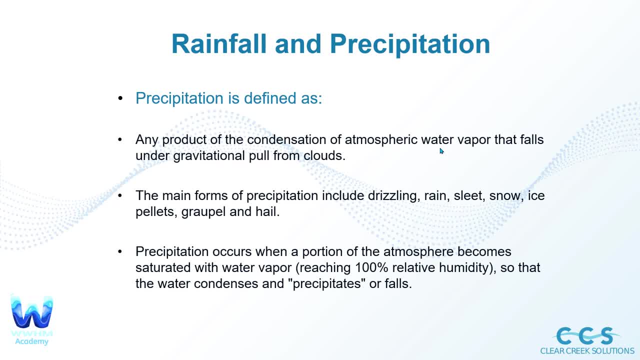 The main forms of precipitation include drizzling rain, sleet, snow, ice pellets a group will inhale. Precipitation occurs when a portion of the atmosphere becomes saturated with water vapor, reaching 100% relative humidity, so that the water condenses and precipitates or falls. 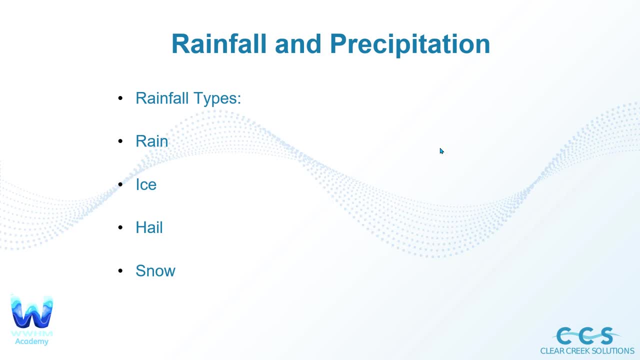 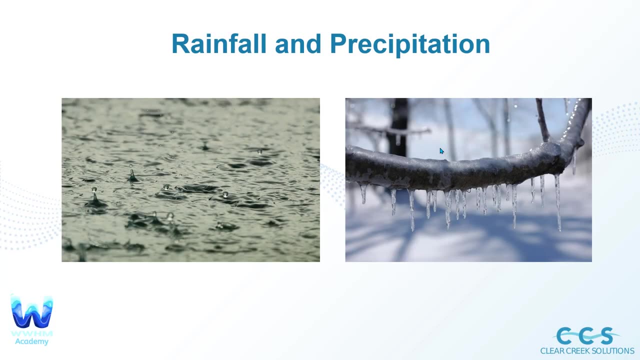 So here's some of the different rainfall and precipitation types that are often identified in hydrology and water resources engineering. We have rain, ice, hail and snow. They're going to act slightly differently, So just to give you an idea, I'm sure you've all seen these type. 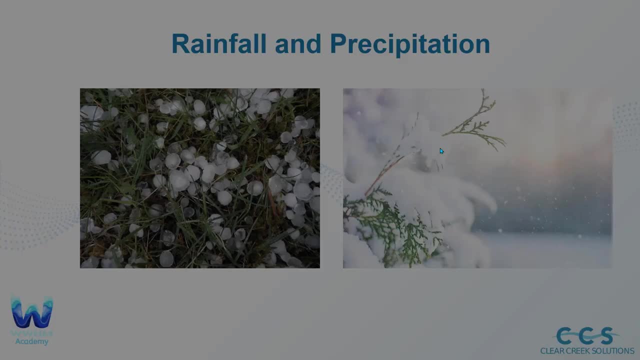 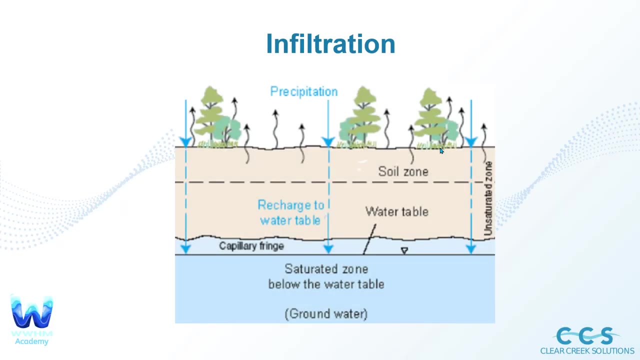 of weather forms, but it's important to point out pictures. We've got rain, we have ice, we have hail and then we have snow, and they all occur under different weather conditions. So what happens to that water when it rains on? let's say it just rains on the ground. Well, that precipitation.